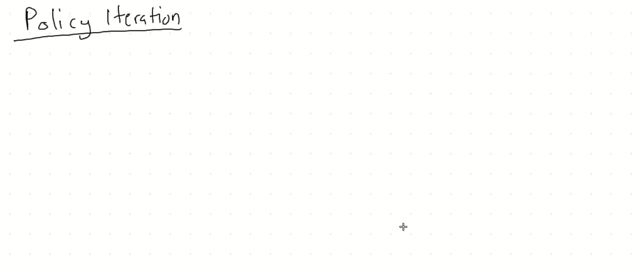 Hello and welcome to our fourth lecture in the Jabra Reinforcement Learning series. In this lecture, we're going to go through our first reinforcement learning algorithm, known as policy iteration. Now, understanding this algorithm is going to be really important, because this algorithm is the foundation of most of the other algorithms that we're going to look. 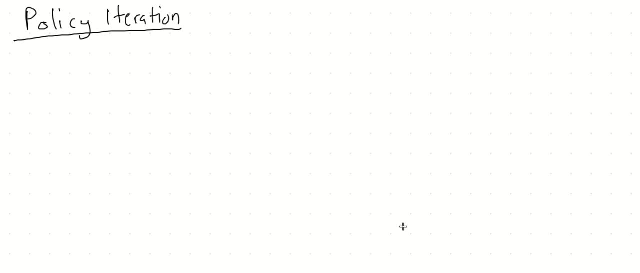 at in the future lectures. So the generalized version of this algorithm actually shows how most of these other algorithms work, and it's important that you fully understand how this one works. So, since this algorithm is the foundation of what we're going to go through in the future, 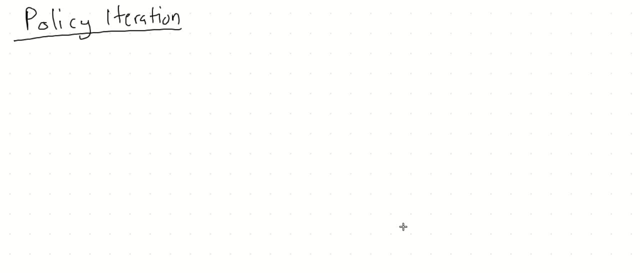 I've decided to split it into three lectures, So we won't just cover this algorithm in this lecture, but the next two lectures as well. So what's important to know about this algorithm is that we split it into two, What is known as policy evaluation. 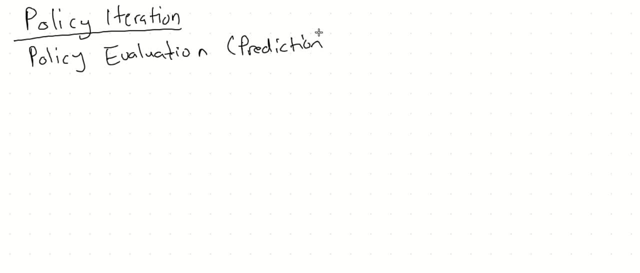 rather prediction and policy improvement, what we know as control. So this lecture is actually going to be focusing on this: the policy evaluation, The next lecture. so this is for the next lecture. The next lecture will be focusing on policy improvement or control, and finally the lecture after that. we'll kind of combine these two to get our policy. 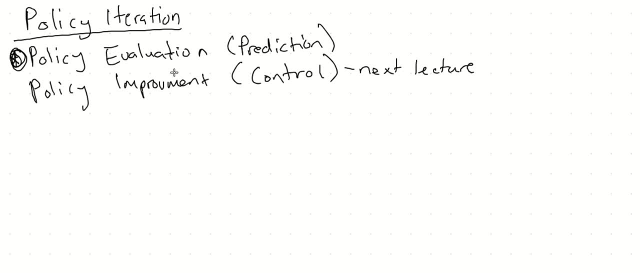 iteration algorithm and we'll even go through the generalized policy iteration concepts behind understanding how reinforcement learning algorithms work. So let's start with policy evaluation Now. we need to do this with an example, for, to make it easier for you and if you remember, from our very first lecture, we say that our 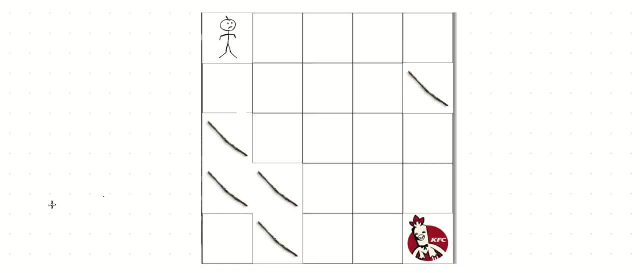 ongoing example would be this one here. So if you remember how this was working, we have this kid who will store money from his parents. So what this kid is trying to do is is navigate this maze and trying to reach where we've got the kfc, uh, where you can go buy kfc. 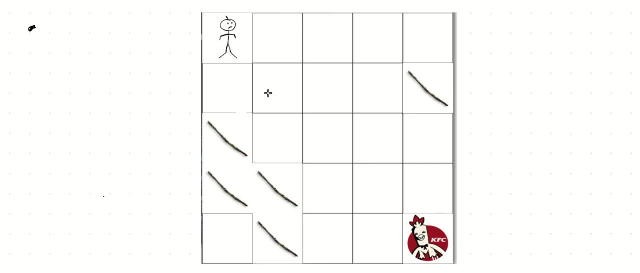 with the money he stole, but he needs to avoid getting caught, because if he gets caught, he gets a beating, essentially. so all these areas where there's sticks right- uh, all these states actually the. these are the areas where the kid will get caught and the game is over, or whatever this. 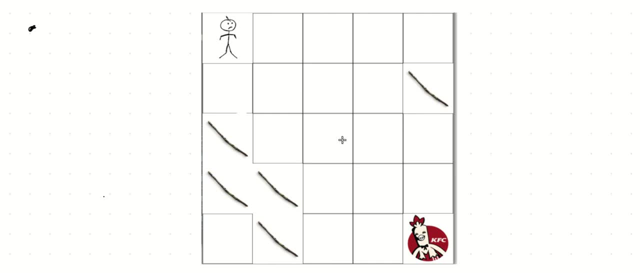 scenario is over. but if he reaches the kfc, he achieves his goal, and so forth. so, if you remember, we need to go through some of the things like: what is the state in this scenario? well, the state is essentially where the kid is at right. so if he starts at this point, we call this. uh, let me use 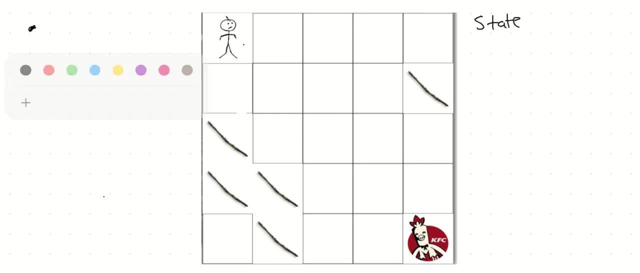 a different color for this. okay, so we call this you s zero, right? that's the, let's say, the initial state the kid can be in and at time, step one, the kid can either be here or he can be there. so let's just give this kind of like a very generic 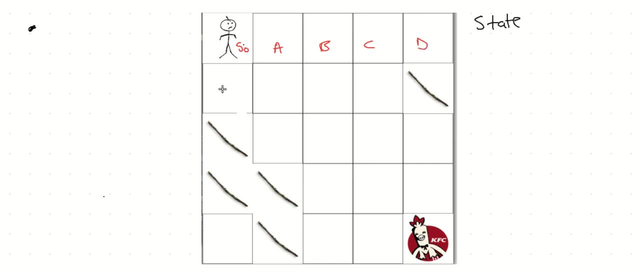 descriptions: a, b, c, d, let's say e, f, g, h and so forth. so all these letters, so the state space comprises of, like uh s, zero, which we call the starting state, and then we've got a, we've got b and so forth. right, this is actually. 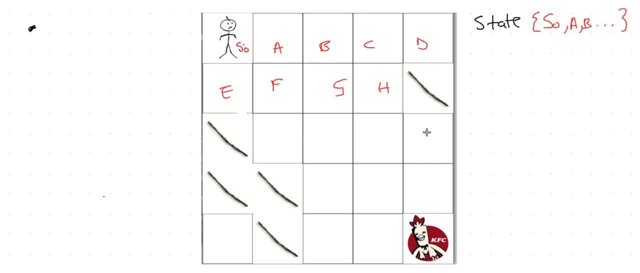 what our states are in this simple environment and, uh, what are the actions that the kid can take, right? so what are the actions? let's look into that. what are the actions that the kid can take in the states? so essentially he can take is move right, move to the left, move up and move down right. that's how he navigates this. 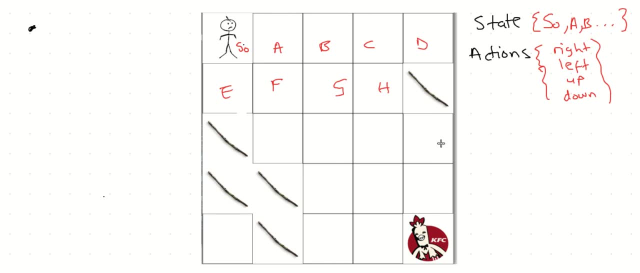 maze. these are the possible actions that this kid can take in this kind of scenario that we've described here. so now that we know what the state are, what the actions are, the next thing we need to know is: what is our goal right? so if the kid was returning to the space? so from the last lecture when we looked at goals and rewards, 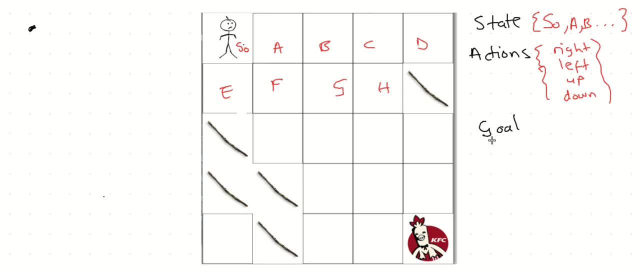 if you remember, the goal was to maximize the return, right? so think for a second like: what had we defined the return as so? essentially, the return is the summation of all possible rewards that the kid will get as it's going through this maze. so let's assume 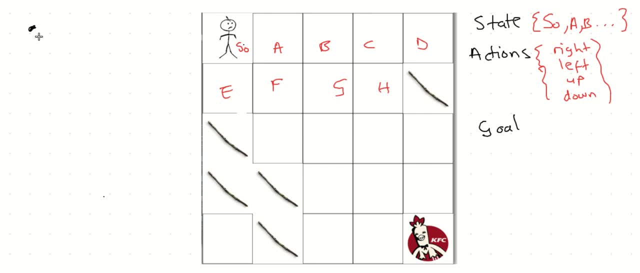 we know the dynamics of this environment. right, we're gonna keep itữail意. We are going to keep it really simple for this case. So every single time this kid moves from one state to another, he moves either there or he moves there, depending. 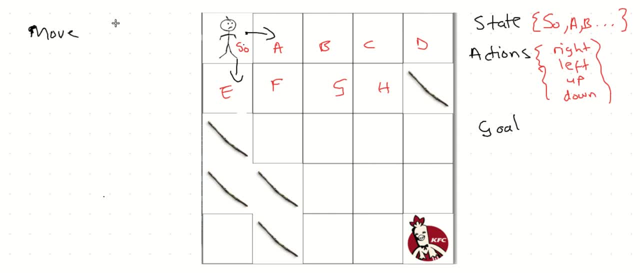 So every time he moves he gets a reward of zero. nothing happens. And if the kid ends up in this state, where there is a stick, so this is. if he moves, so this is the reward. sorry, he ends up where there is a stick, then he gets a reward of. 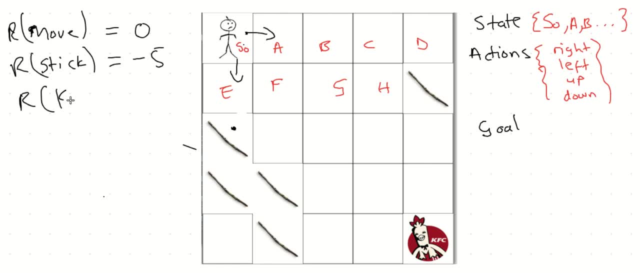 say, minus 5.. And if he reaches his goal he gets a reward of minus 5.. And if he reaches his goal he gets a reward of minus 5.. And if he reaches his goal he gets a reward of plus 10.. 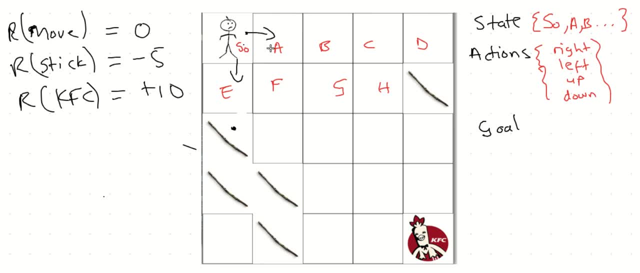 So the idea is to maximize the reward, and to maximize the reward, you just need to find the series of actions that will lead you to the state where you've got your KFC. So that's how we define our rewards, like this. So right now, it's not important for you to really. what's important actually is for you. 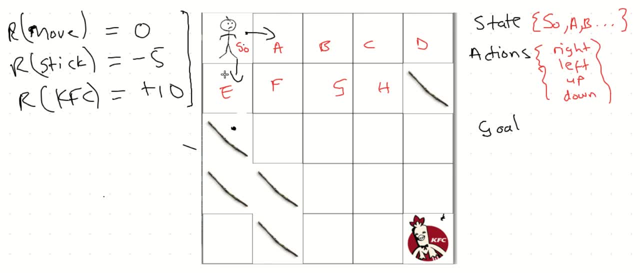 to just know that. ah, okay, every movement, you get no reward. So if you reach this, where there's a stick, you get a negative reward. If you reach here, you get a positive reward. That's essentially what we're showing here. 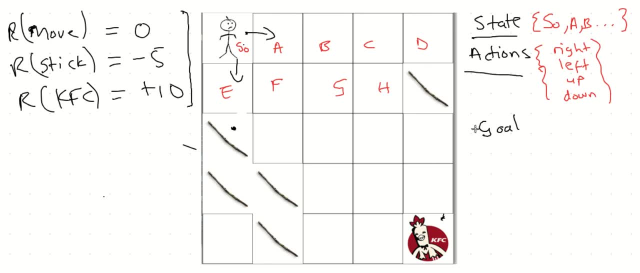 And we are showing what the state is, what the actions are. And now, what is our goal? Our goal is to maximize the reward right. So the goal is to maximize, say, the accumulated rewards. So what this means is. So what this means is: 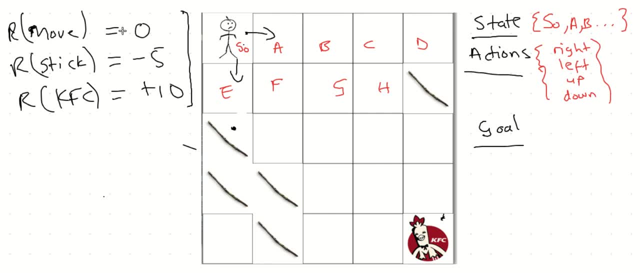 Like we had a different version of this problem Here. we defined our move as 0. But maybe we might define our move as minus 1.. So that means the kid has to find the fastest way to actually reach this goal So that he doesn't lose a lot of points for every movement that he makes. So, depending on the kind of problem you want to solve, maybe you define the reward as 0 because you don't care about the amount of time it takes to reach the KFC. He just wants to reach the point. 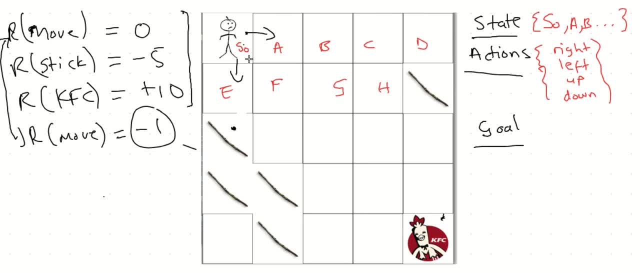 Or you define it as minus 1, where you go like, oh okay, I need to get there as fast as possible. So your reward definition is actually what's going to help you And it's going to affect how you actually navigate through this environment. So our goal is to maximize the long term cumulative rewards. 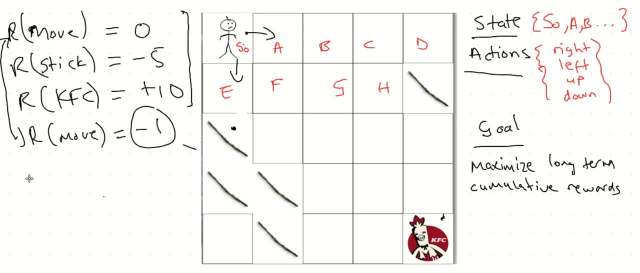 Right, This was essentially our goal, Or rather to maximize what we call the return GT, which is equal to, if you remember from our previous lecture, RT plus 1 plus gamma, RT plus 2 plus gamma squared RT plus 3.. 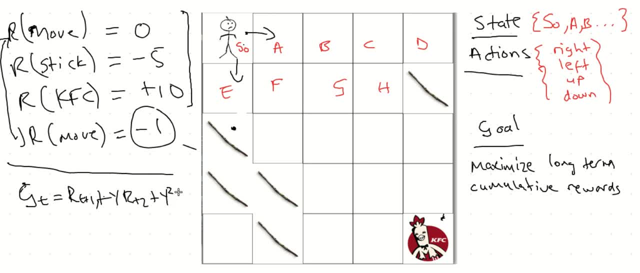 Let me write this more clearly: Gamma squared, RT plus 3 and so forth. Right, This is how we had returned. This is what we actually want to maximize. So we have this kind of definition. Okay, You have a basic understanding of this environment. To reiterate, you are in the state, and these are the possible states you could end up in. 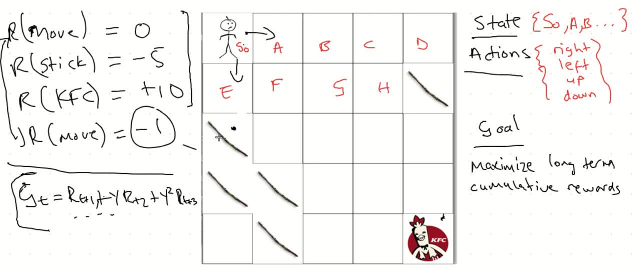 And these are the actions you can take, And this is the goal, And this is the return, And these are the rewards you can get. So here, what you're just supposed to understand. don't focus on this example particularly, but just get the idea of 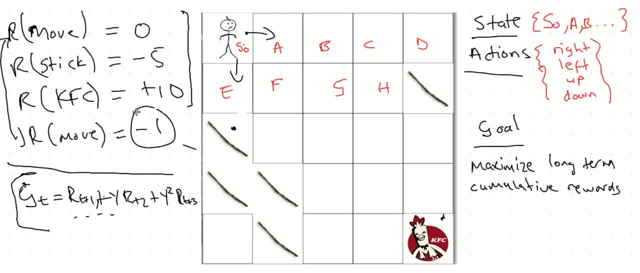 Whatever problem you're trying to solve, you're in a certain state, you need to take an action, and each action will lead you to another state with a certain probability, which you should know if you're following our previous videos- And the goal is to maximize the long term cumulative rewards, Right? So, now that we've described the scenario, the first thing we need to actually define is what we call the value function, Right? So? 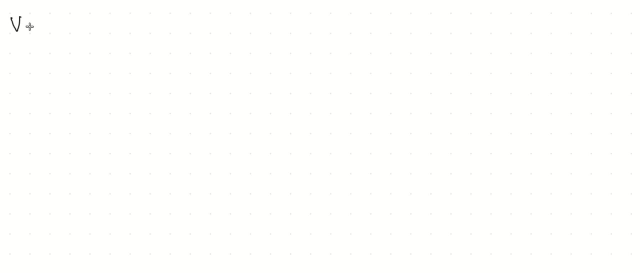 Let's move On to the value function Right. So what is this value function Right? We define it as V of S, Right, Where S is a state. So V of S is essentially saying how good is it to be in a particular state, Right. 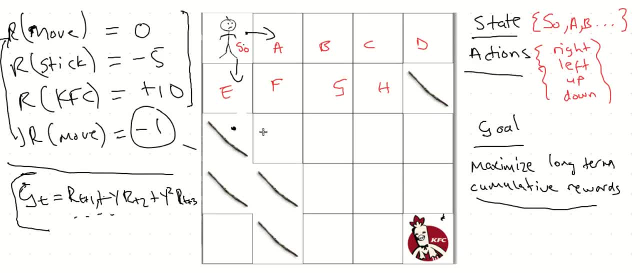 So if we go back to our example like: what's the value of the state? What's the value of the state? What's the value of the state? So let's say we say that the value of the state is 10.. The value of the state is 8.. This one is 8.. This one is 6. And this one is 5. Or this one is 4. Or whatever. So if you're in this state right here, this is where your agent is. let's say: 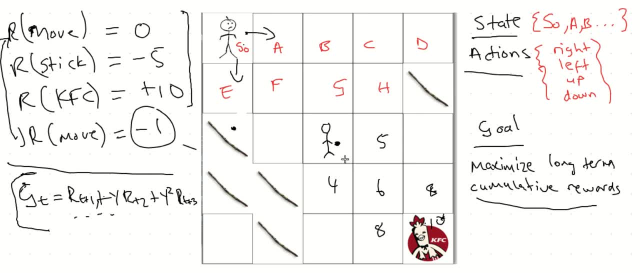 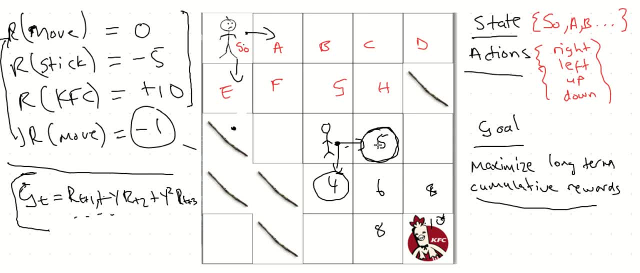 state is a value of five and this one is a value of four. so you know that it's better for me to be in this state. so you'll make a move to go into this state, right, and from here you go like, okay, let's say this is a value of, say, four again, oh, okay, it's better for me to move down there. 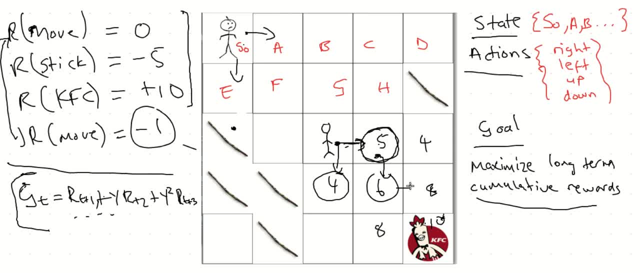 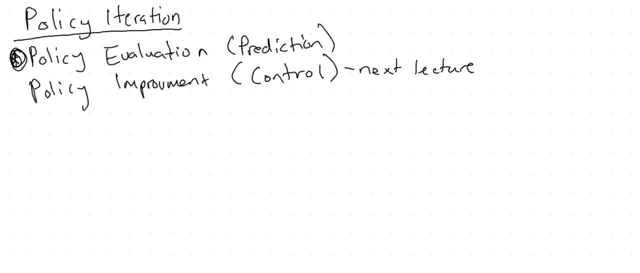 and here. whether i move here or here, it doesn't make a difference, and finally you reach there. so your value function actually gives you an idea of where you actually want to move, based on how good it is to be in a particular state. okay, so if you understand that, this is how we define vs right. 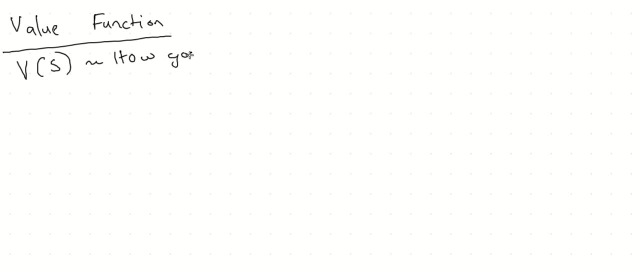 so how good it is to be in a particular state. right, that's what our value function is, and the next thing we actually need to know is: what is policy right? so we denote a policy by pi right, pi of s right. so what is pi of s, you might ask. well, this is what action to take. 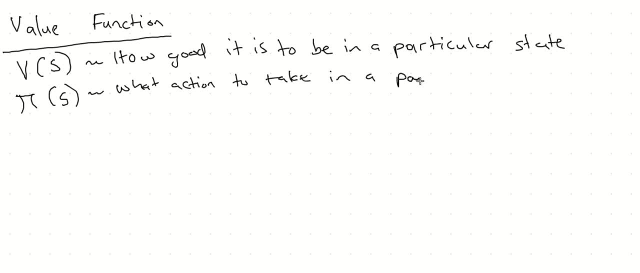 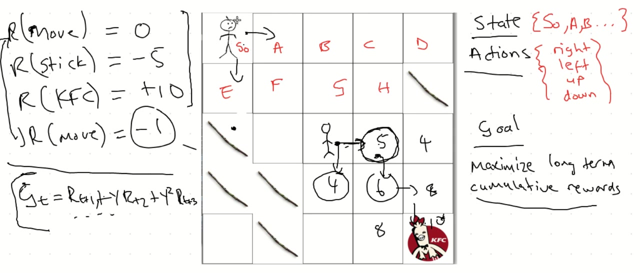 in a particular state, right? so this pi of s gives us, uh, information of what in what action are we supposed to take? we denote this pi of s. so again in our example here, if we are in this, uh, let's say, initial state, here we're in the initial state and we say: what is pi of s there? 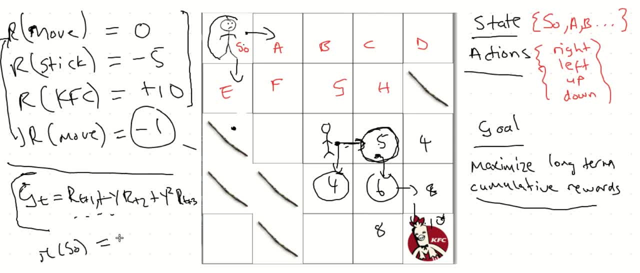 right and someone say pi of s0 is equals to right. okay, that means that the policy state: if we're in state s0, we should move to the right. and then pi of this a is equals to maybe if we're here, we want to also move to the right, this will be right. and then pi of uh and so forth. that's basically. 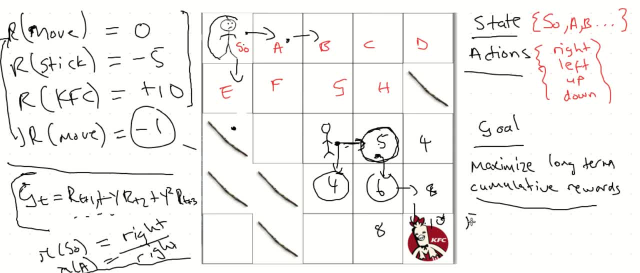 like how it's working, like if we say pi of of course, b again is to move in a certain direction, and so forth. uh, this has become too cluttered, so i'll just leave it at this. so that's what pi is. it's just a function, a function telling us. 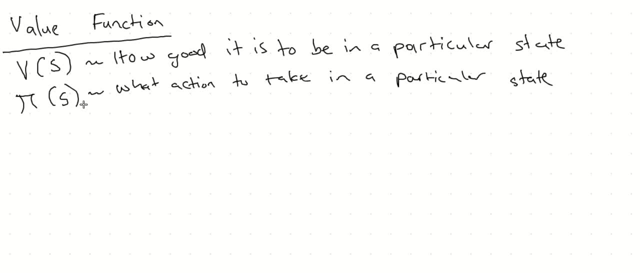 what to do in a particular state. so please know the difference between the value function and the policy. the value function just tells us how good it is to be in a particular state, and the policy is a function telling us what action to take in a particular state. right. 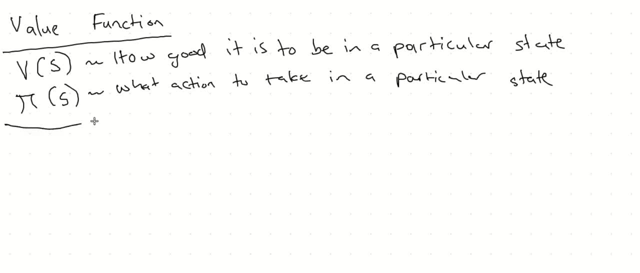 so if we have an understanding of what those things are, then we are actually going to look at something, uh, called v pi of s, right? what is this now right? that's what you're probably going to ask yourself. well, v pi of s is essentially saying: using 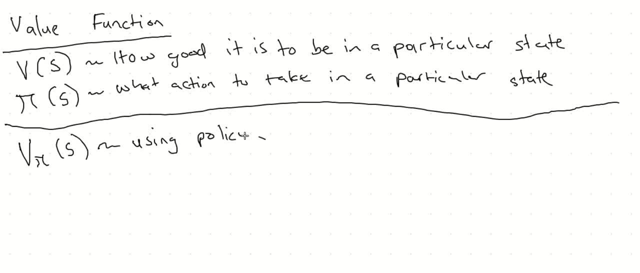 policy, pi right using this policy? what is the value of state s right? so if someone gives you a policy, like by saying, give you a policy, is just telling you that in every state, uh, you're supposed to perform a particular action. so someone gives you this function right. 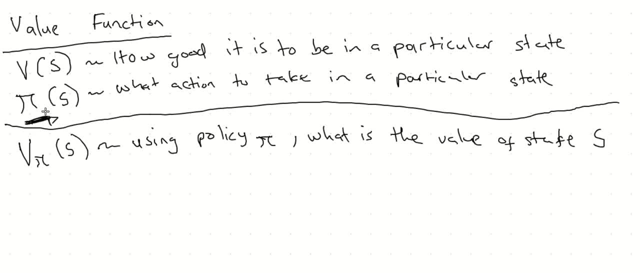 uh, it's in the future video that we're actually going to go through how we estimate this function, but for now let's just say: someone gives you this function and now that you have this function, you are supposed to calculate. right, you're supposed to calculate the value of being in. 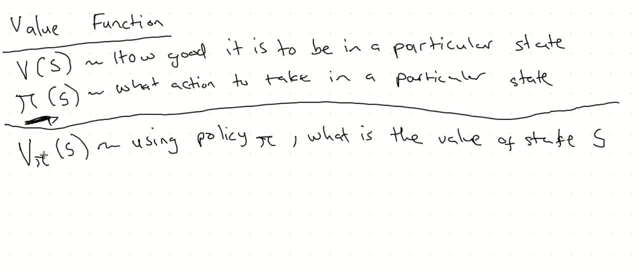 a particular state, given this function right. this is what we call v pi of s right. so you're given pi right and you're trying to find the value of being in each state under the given policy. okay, that's the idea here. so, under the given policy, you're trying to find the value of being. 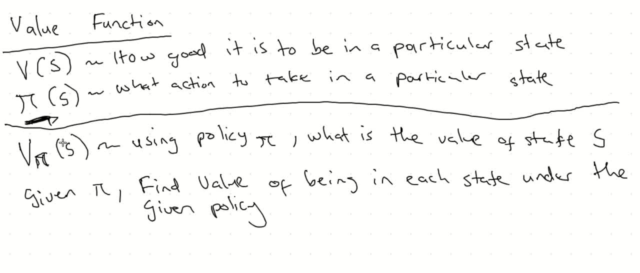 in each state. uh, that's what v pi actually ends up being here. so we are going to assume right now that we're given pi and we're trying to find the value of being in this state, and this is what we call the prediction problem. right, this is the prediction problem. 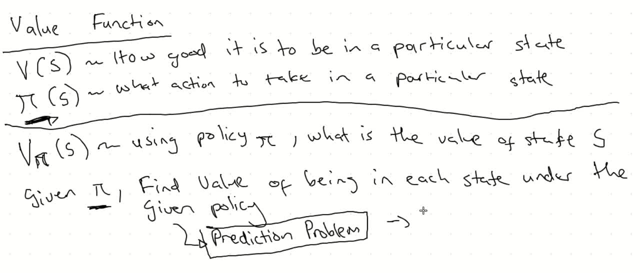 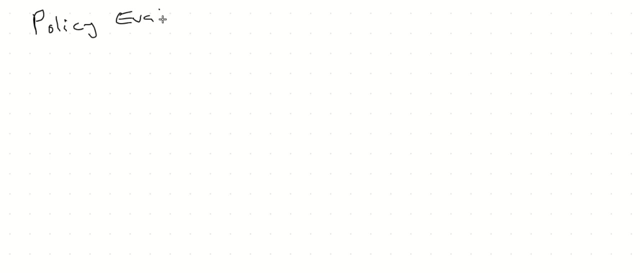 this is the prediction problem, also known as policy evaluation, which is the main subject of this lecture. actually, the main subject of this lecture is policy evaluation as such, so let us start on the policy evaluation algorithm now. for you to understand this, make sure that you've actually gone through our previous lecture. 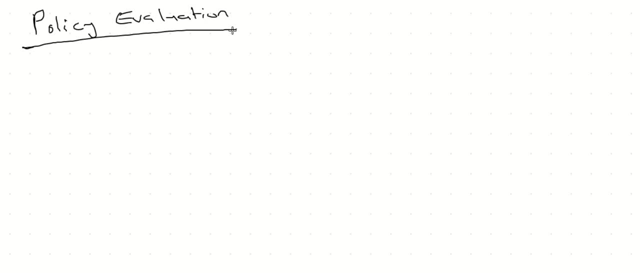 because you'll need to know what transition probabilities are, how they work, and so forth. so let's start again. so what is again v, pi of s? we've already gone through this. we have been given pi and we need to estimate the value function of s. so how good it is to be. 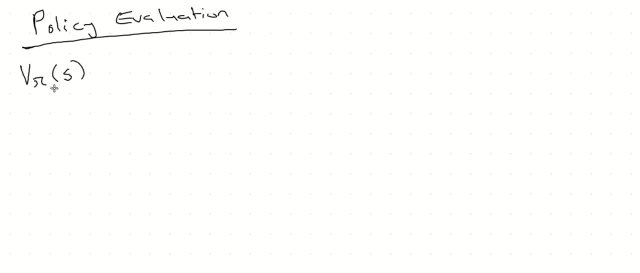 in state s and the policy pi right. well, this is actually equal to the expectation, right under policy pi, of the return gt given s. so, of course, like you might wonder to yourself, like, what does this actually mean? right, what is this? so we defined the return as the accumulation. 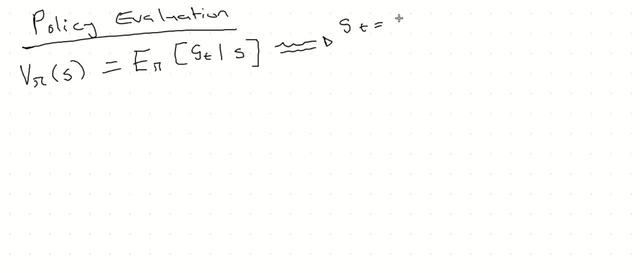 of discounted rewards. so i'll just rewrite the formula here: rt plus one plus comma, rt plus two plus comma, squared rt plus three and so forth. right, this is how we defined the return. so, given this definition for the return, we are actually trying to now say that, well, we don't know what rt plus one, we don't know what rt plus two is, rt plus three is. 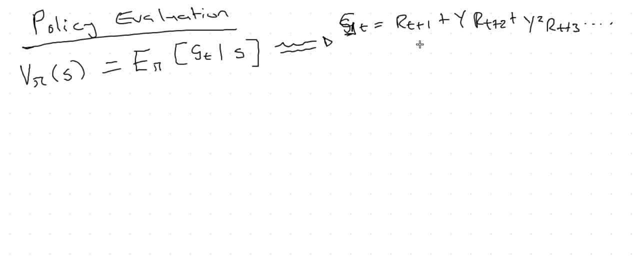 and so forth. so because we don't know where we're going to end up in our series of events. so these are the essentially random variables and since they are random variables, we are going to need to take the expectation right of these variables. so how good it is to be in a particular state, 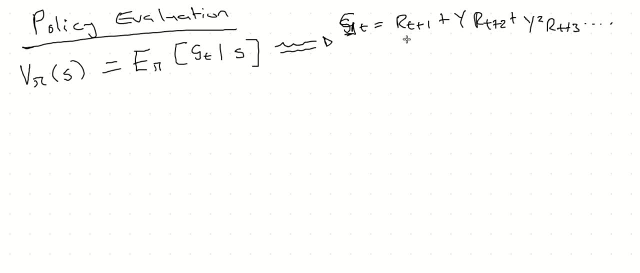 is essentially like: what is the expected reward? what's the expected cumulative reward that we'd get starting from that state? okay, that's essentially how good it is, so if we start from state s. and then what's the expected reward? that's the value of being in that particular state. 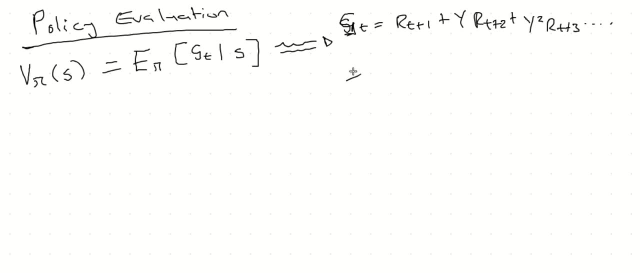 essentially so, given that we can now infer a couple of things here. right, so this is the expectation of $gt given s right, and this is actually equal to the expectation ange policy pi of. we can actually divide this into our t plus 1 right plus gamma. 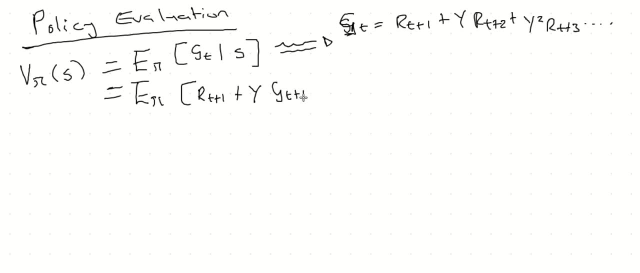 multiplied by $gt plus 1 given s, okay. so if we subtract this from this here and then it will become a equation, right, and so on, until we get $gt plus 1, we will be getting romantic island, right, talking about it all. so you can actually take the expectation of $gt pagina for every component, right, and so on: x, rt6, all right. so this is the expectation of $ jt given s and this is actually equal to the expectation and a policy pi of. we can actually we can actually divide this R T plus 1 rightjackChozaz in R T plus 1 right來en. 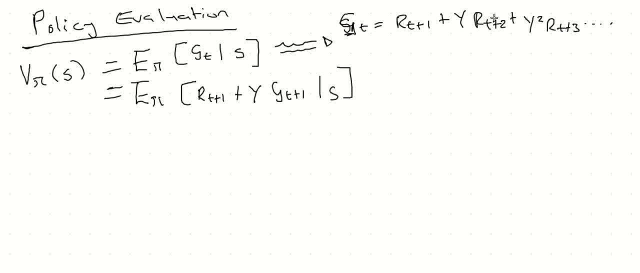 Now, why is this the case? Because all of this here. well, if this is rt plus, if this is gt, then obviously if gt is rt plus 1 plus gamma times some function. that means, if we start from rt plus 2 here, this is actually signifying gt plus 1, right? 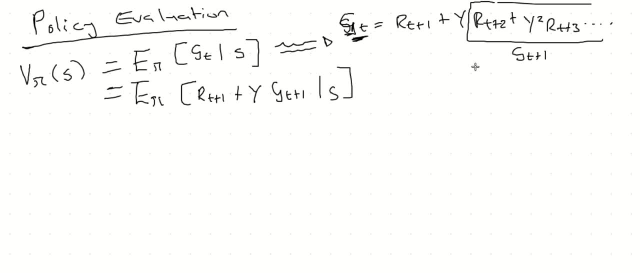 That's the idea here, So you should convince yourself why this is the case, But I think it should be simple enough to see from you. Okay, So now that we know what all of this is, we go on to the next problem. 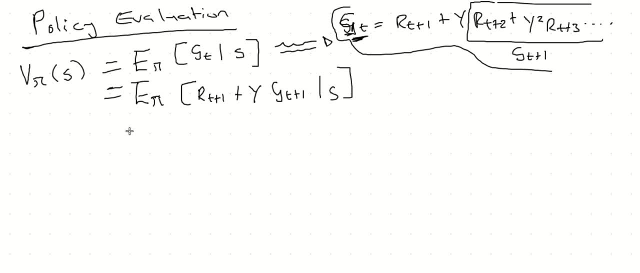 So we've broken down this equation like that. We can break it down even further by saying this is the expectation under policy pi, the policy that we've been given, of rt plus 1 plus gamma right, V pi right S, t plus 1 given S. And why is this the case? Because we said V pi of S is the expectation of gt right. 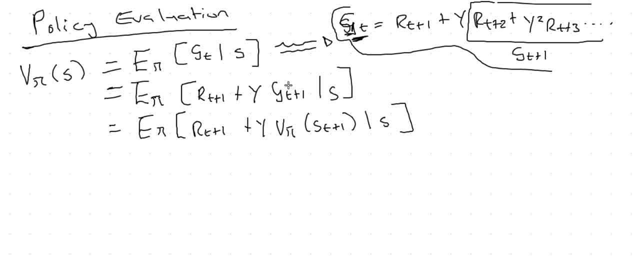 So how good it is to be in a particular situation. So we can actually replace gt with V pi S t. So gt plus 1 can be replaced with V pi S t plus 1 in this expectation. So we can break down this even further now, right. 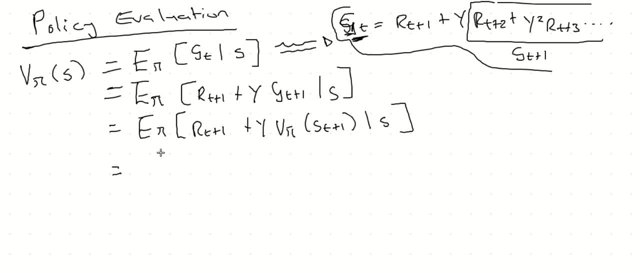 By saying this is actually the. now we're breaking down the expectation To the summation over all possible actions of pi A given S. I'm going to explain what this actually means. right Times the summation over all S prime comma r of P S prime comma r given S comma A. This is our transition probability. 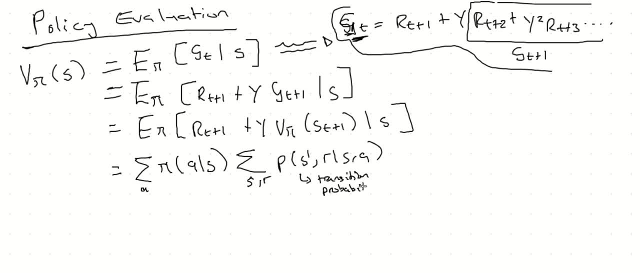 This is transition probability. Let's look at this: Multiply by r plus gamma, V, pi of S prime. right, This is actually the summation over S prime, sorry. So, of course, now you're probably wondering like: how did we actually get to this stage? 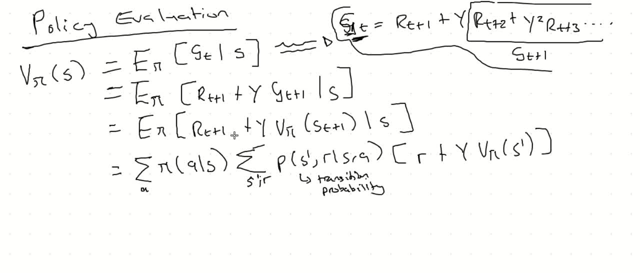 Like we actually get to this stage by dividing by r, So we get to the end of the equation. we actually just broke down this expectation. So let me break down these terms one by one. Let's start with this term here, This term over here. So what this term is saying is: 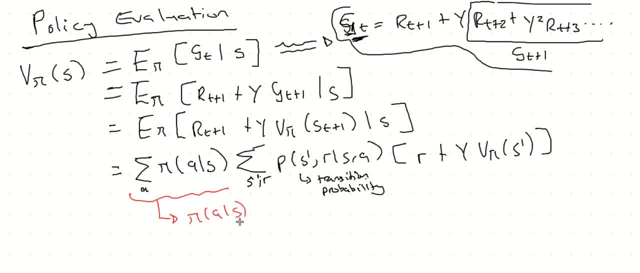 summation of Pi A given S. So if you remember, Pi A was actually supposed to be the positive policy that we take in a given state. Sorry, Pi S was kind of like what action should we take in a given state? But sometimes this action can be a probability distribution. 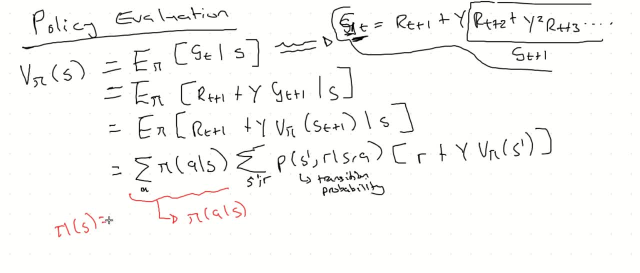 So this is essentially like: okay, this is equal to some action you should take. But if you are now given Pi- sorry, if you are now given Pi- this is essentially like: okay, A given S. that means A is taken, action, A is taken with some probability, Right? So 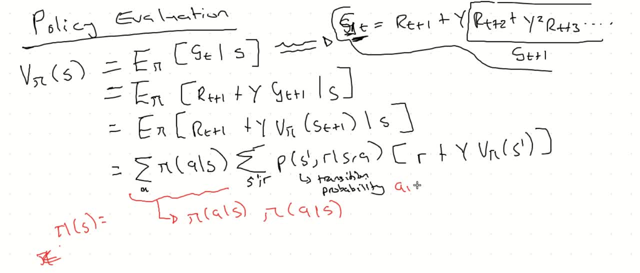 if we can take action 1 with a probability of- sorry, let me clear this up: Probability of taking action 1 may be 0.2,. probability of taking action 2 is 0.8.. Right, This is given that you're in a particular state. 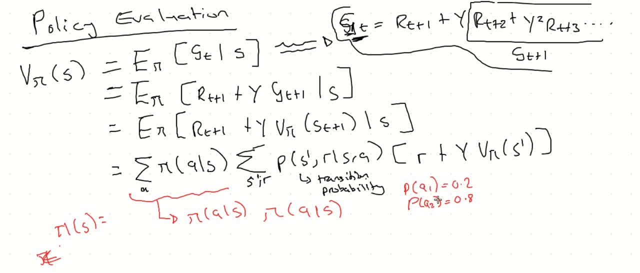 So this is actually probability of A1 given S, probability of A2 given S. So this is essentially saying that pi of A given S the probability of taking an action in a given state. That's what this is right. So that means that the action that we take in our given state 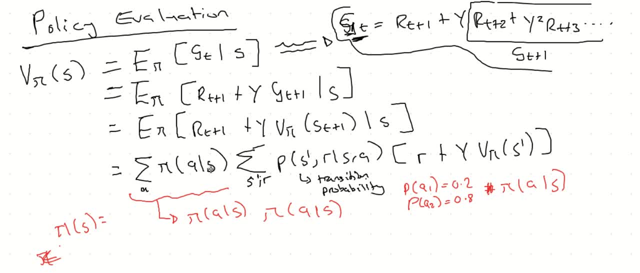 is not always certain. We might take different actions with different probabilities. Now, this is the transition probability. You should know what it means. The probability of ending up in some future state S' R, given that you're in some state S and you take action A. 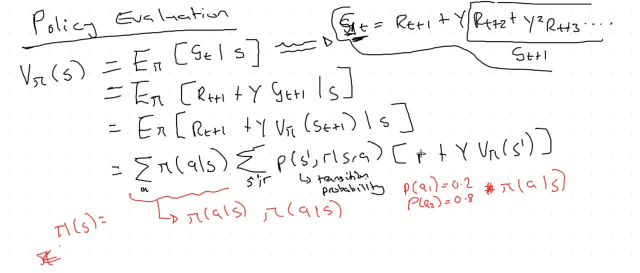 And this is the reward that you get for taking that action, plus gamma times what we have here, which is a value function for being in a future state. So I know, right now this is most probably not clear to you, and that's perfectly fine. I'm actually going to explain using something that we call a backup diagram. 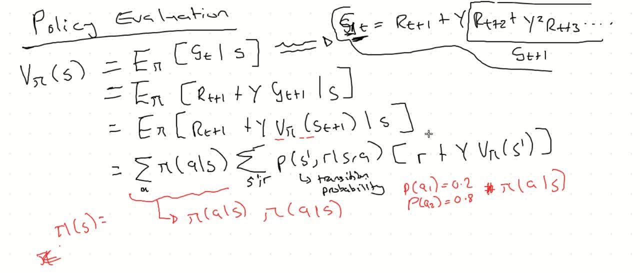 and this should clear all your doubts, and it's a different representation of what this actually means. Of course, you can actually work through in your head right now. You can pause the video and think about why this formula leads us to this position, But 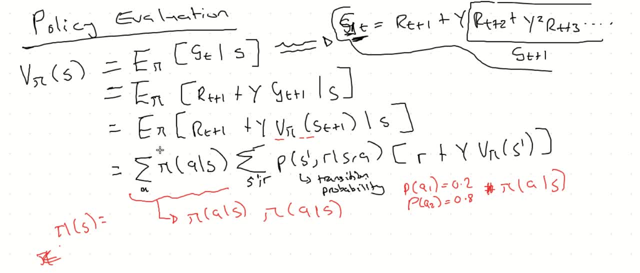 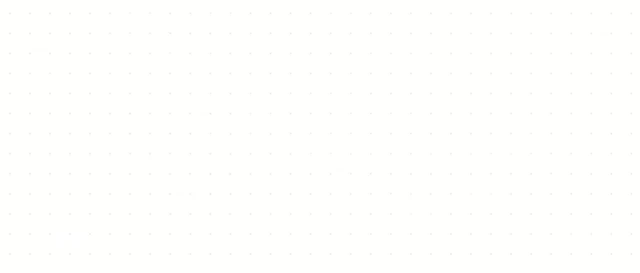 right now. I'm going to make it even simpler by looking at this formula using a backup diagram. Okay, So let's do that. Oh, sorry. Okay, So we're going to start with. okay, let me go back to our traditional black. 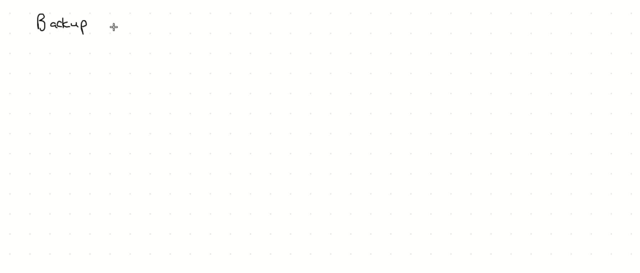 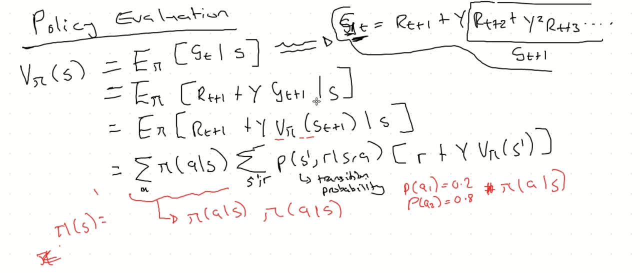 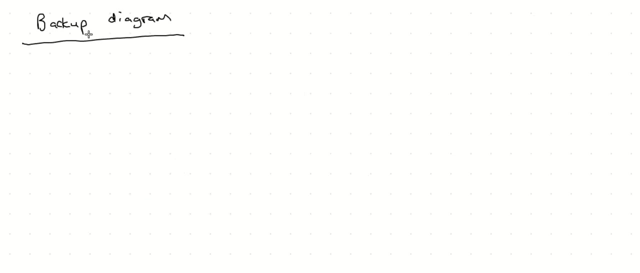 with a backup diagram so that you understand. this representation we showed here was for those that are more like into the math and the statistics of how it's actually working, But this diagram should help you visualize actually what's actually going on as such. So let's start with our backup diagram. 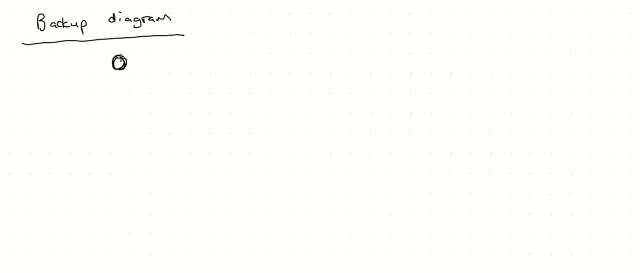 and we start here. Okay, In a state S. Okay, So from this state we can take an action A1 or a different action A2, or another different action A3.. I hope you can follow right. So from given state S. 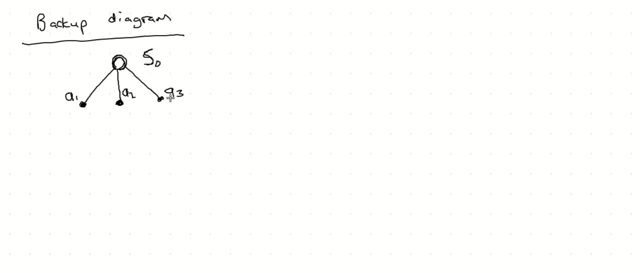 I don't know S0, we can take actions A1, A2 or A3, right? So we define pi of A, given S0 to be the probability that you take a particular action from state S0. So we can have: 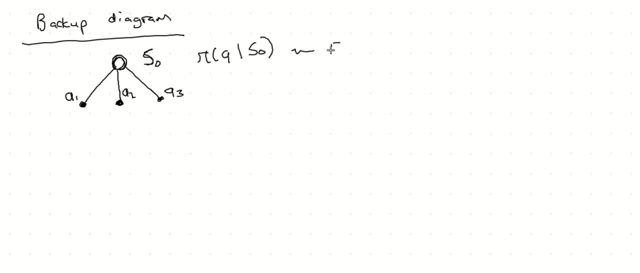 some kind of definition like: okay, the probability of me taking action 1 in state S0 is equals to, let's say, 0.2, the probability of me taking action 2 in state S0, maybe this is 0.5,. 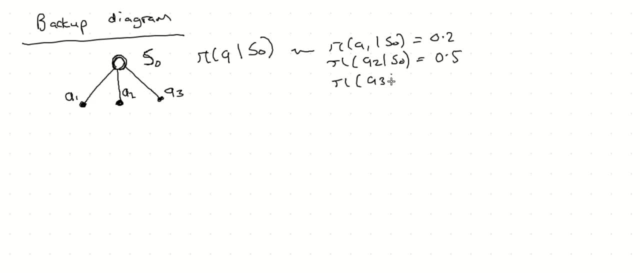 and the probability of me taking action 3 in state 0, maybe this is equal to 0.3, right? So we've broken down those probabilities, right? So that's what this pi A given S 0, actually means, okay. 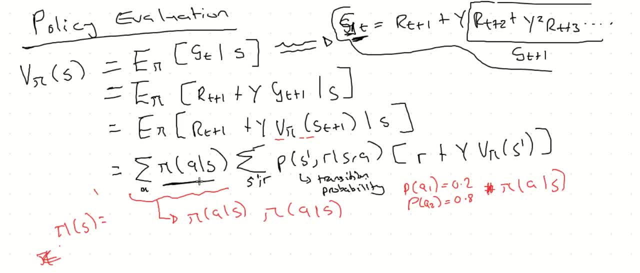 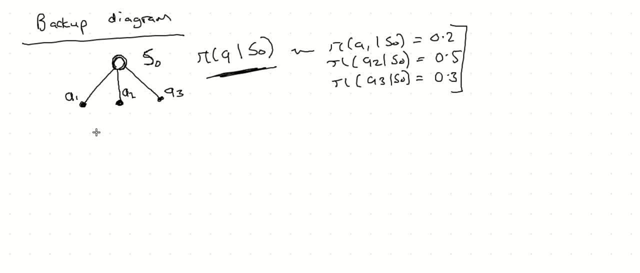 So this should help you understand what this term is. okay, Okay, sorry. Now, if you take any action right, You might end up in a new state S1X, with some probability, Let's say you take action A1,. 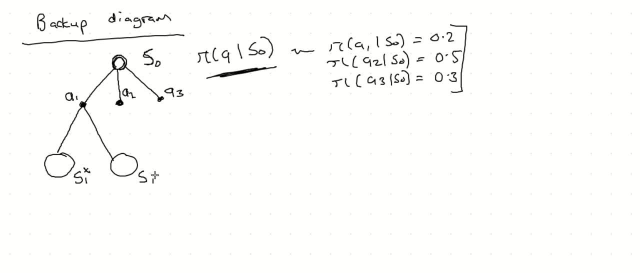 or maybe you might end up in some other state S1Y- with another probability. If you went through our previous lecture, you should be able to understand why one action can lead to different states, right? Please see the previous lecture in case this actually confuses you. 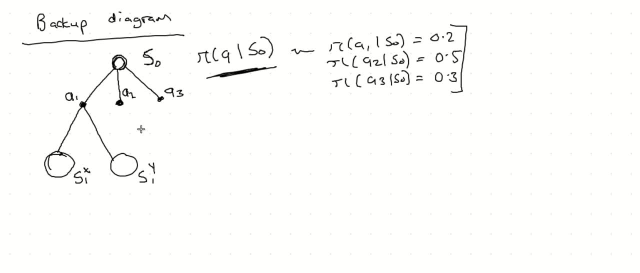 So what does this actually mean? It actually means that, okay, we have a probability of ending up in state S', where S' can be S1X or S1Y, right, Getting some reward, R given right that we're in some state S. 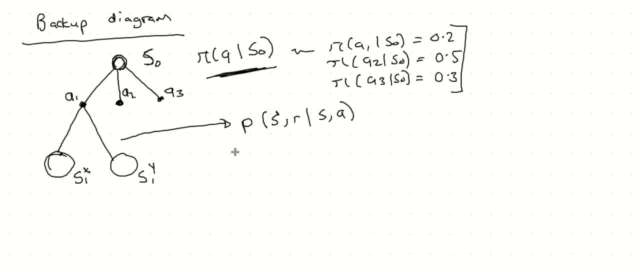 and take action. A right. This is what it is. So for simplification, we will abuse this notation a bit and just represent it as S' given SA. So these two, you can just think of them as interchangeable, because in most of the times, 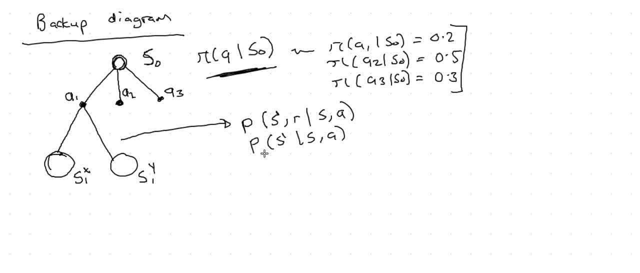 these are associated anyway, So the probability of ending up in some state S' given SA. So these two are interchangeable, Changeable right. So I can either use this one or this one, just depending on things. So what we have here is that. 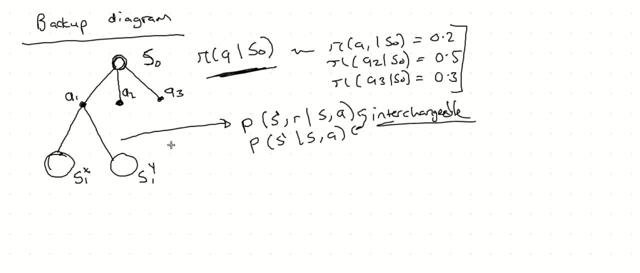 the probability of ending up in S1X right, given that you're in S0, is that you want to express a certain follows that you're in S0 and you take action A1. That's what this line here is representing. 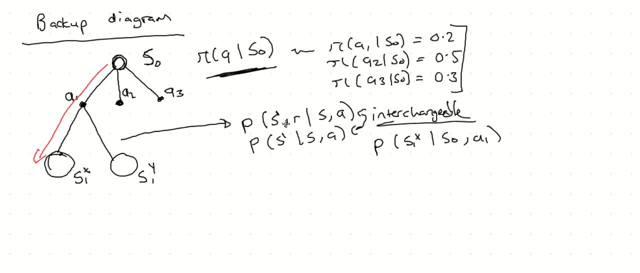 The line that you see here, the chain of events that goes up to here, is actually representing this: the probability of ending up in S1x, given S0, A0. And the other chain of events, the one we see here, going down there. 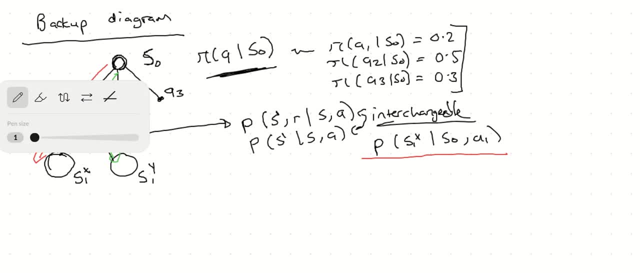 what this is essentially is the probability of ending up in S1y, given that you are in S0 and you take action A1.. That's what this is. So we have these two probabilities that are essentially represented by this here. What that means is that you start in S0, right? 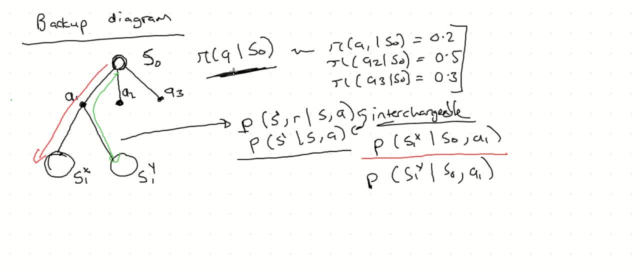 You take an action A1, right, with some probability. okay, The probability of you taking action A1, given you're in S0, is supposed to be 0.2.. After taking action A1, you're going to get a reward, of course, right. 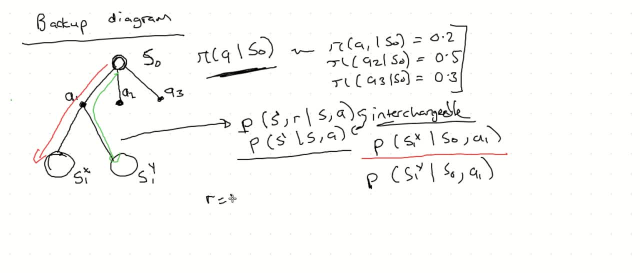 You're going to get a reward R. This is your reward, And after getting this reward you'll end up in some future state S prime right. This is something we've gone through in the previous video, So, again, we're just now representing it using this thing known as a backup diagram, right? 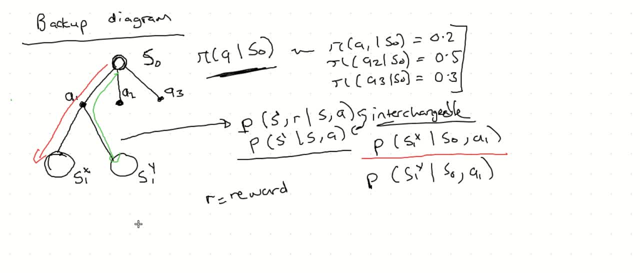 So what does this actually mean? Well, we can actually break it down even more back to our formula. So what is the value Of being again under some policy pi, of ending up of some state S right? This is kind of what we want to compute. 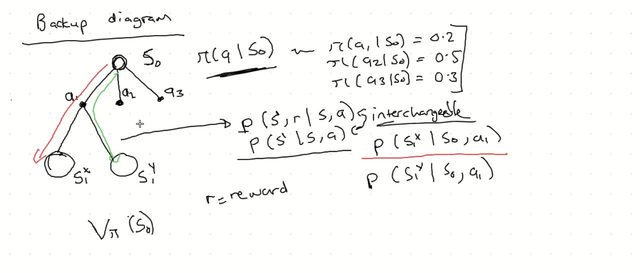 The value of being in S0, essentially, What's the value of being in this state here? That's what you want to know: the value of this state. So the value of this state is essentially equal to the summation over all of the actions, right? 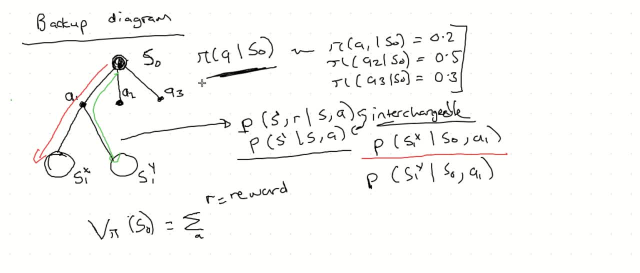 All the actions that we can take in this state, right, Because this is again an expectation. So, since it's an expectation, we're going to consider this probability and this probability and this probability and sum over all of them, right? 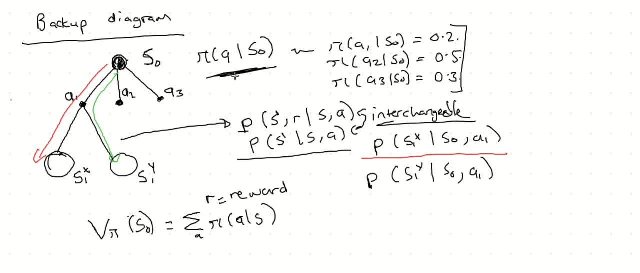 So of A given S, which is what we have here, because we might take any of this action right. That's what this is representing. And then, once we take action A, we'll get some reward right. So we'll get some reward R. 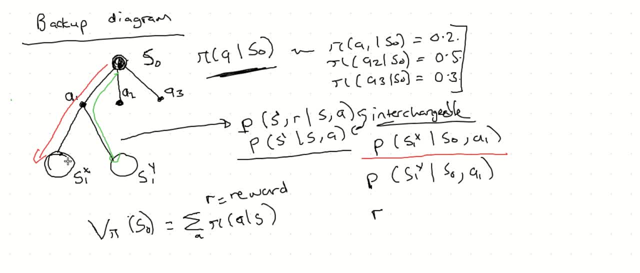 and end up in the state S' right. So plus gamma, end up in the state sorry. plus gamma, the value of S'. So this is going to be the value of S' plus the value of the future state that we might end up in, okay. 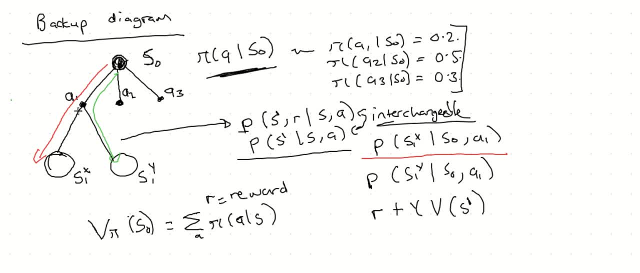 So the value of being here in S0 is the reward I get for taking this action, plus the value of this state, which I don't know yet, but we're actually going to go through how you actually can know what this value actually is. 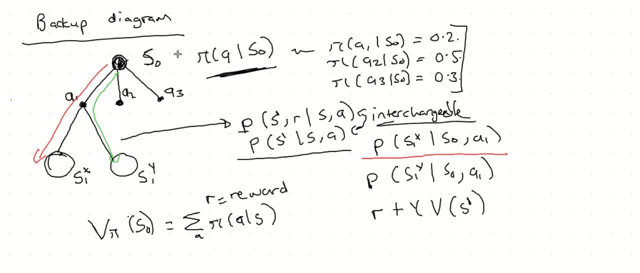 However, we have iterated that this chain of events happens with a certain probability distribution right. So this distribution is again given by the summation over S'R of P, S' given S'A right. So we might end up in this S1,. 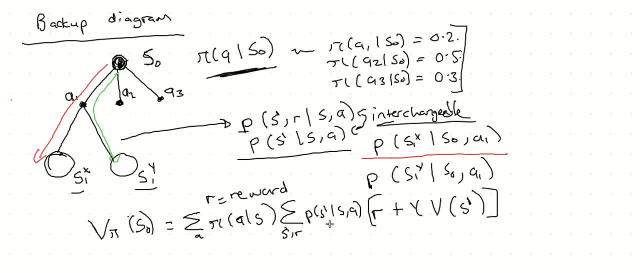 or we might end up in this S1.. Again, another expectation that we're computing here. So that's why we need to multiply the probability of ending up in each of the S' with the distribution of S' reward that we get, plus the value of each of these s primes. again, this is 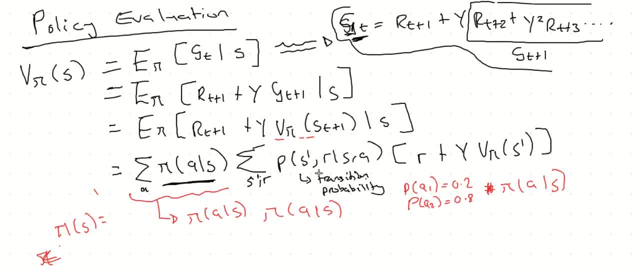 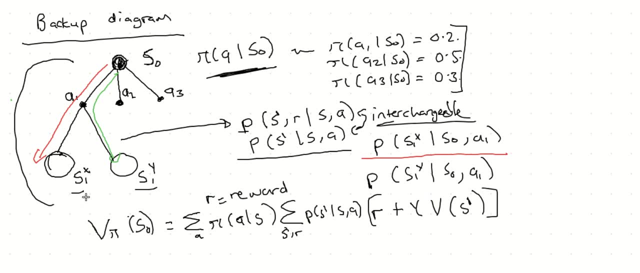 another way of just arriving at the same formula that we saw here, but with a more visual representation of what is going on in this backup diagram. but what you need to actually understand here, what's most important actually, is that, like the way that we arrived here, it might be confusing to you actually at this. 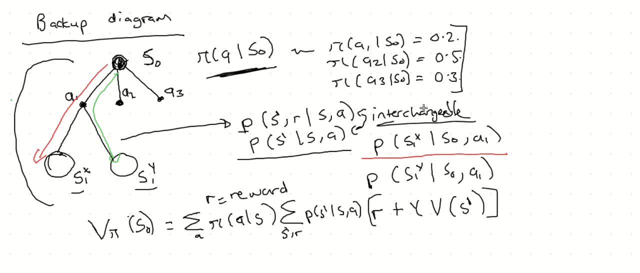 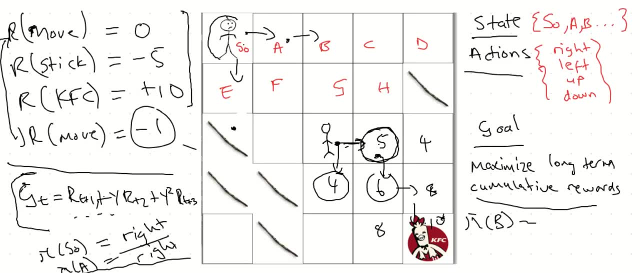 moment, and that is still fine, because we are actually gonna go through a proper example. like when we go through this example shown here at the very beginning, as we were doing, as we're writing our programs, you can actually better see, like, how it's actually working. for now, you don't need 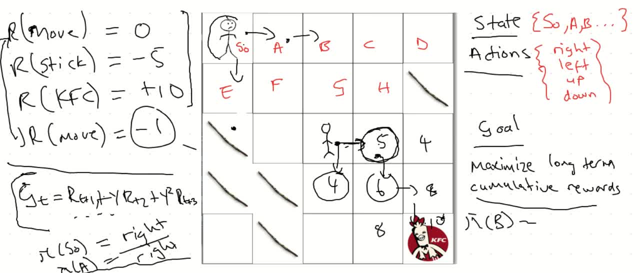 to know how it's actually working. for now you don't need to know how it's to actually get a full understanding of what's happening. but if you did, that's also great, but if not, that's fine, because the example that we're gonna show, like the program that you're gonna write and so forth, should help you, like. 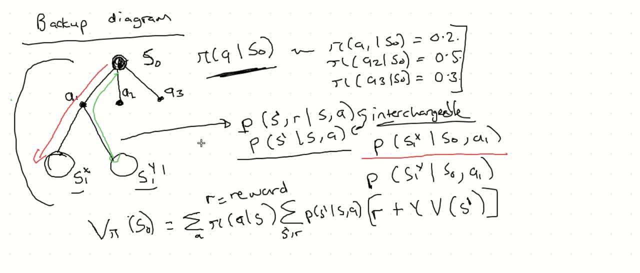 understand how this algorithm is working. so, as such, let's move on. now that we know this is our formula. like, the value of being in state of state as zero depends on the value of being in state as 1x or S1, why? or rather as prime right, and this actually causes some kind of problem. 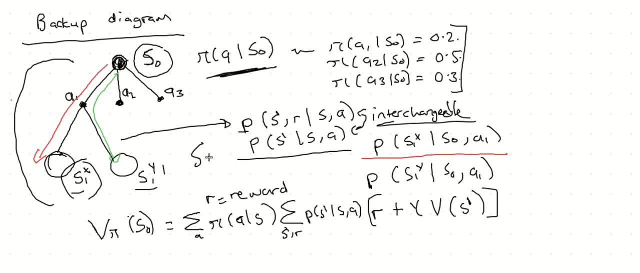 oh sorry, this should be being in state s1, so this causes some kind of problem. we're trying to estimates the value of being in s0- 0 by looking for some value of being in the state of S1, and we have to find a way to do so. 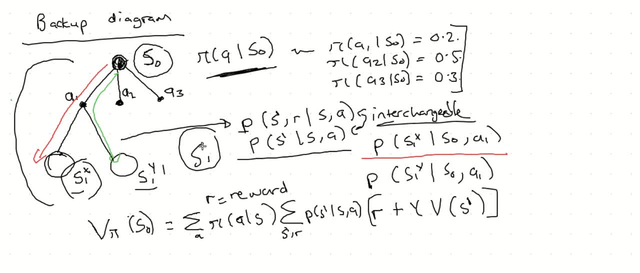 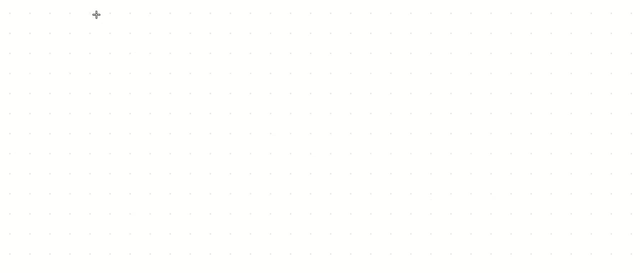 at the value of being an s1, a future state right. well then, that means that we kind of have to iterate right to in order to actually get what this values actually are, and I'm gonna show you what this actually is, maybe from a programming point of view. so what is the value? what is VK right plus 1 of s here? 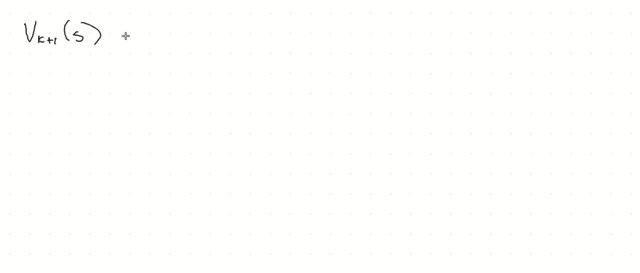 we're defining what is essentially our update rule. so the value of being in state s at time, step K plus 1, right. well, this is essentially the again the expectation of a PI of RT plus 1 plus gamma, VK, st plus 1 given st. this is actually essentially the same. 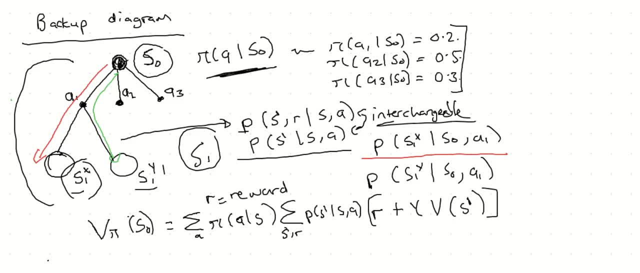 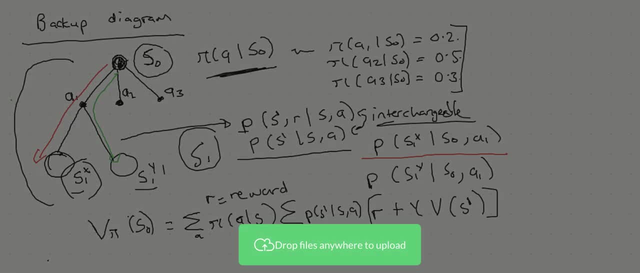 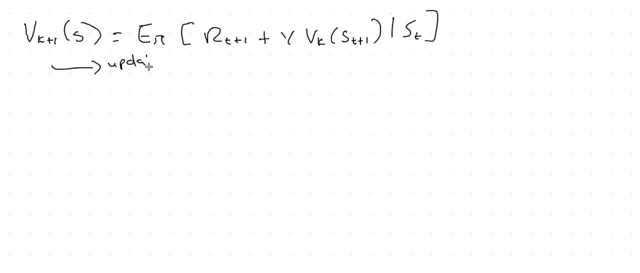 expectation that we had here. sorry that we had over here. we're just representing it using time steps. okay, this is our update rule, essentially, right here. this is our update rule. we can also represent it as summation over a of PI: a given s summation over s prime comma R of probability of s prime given s comma a. 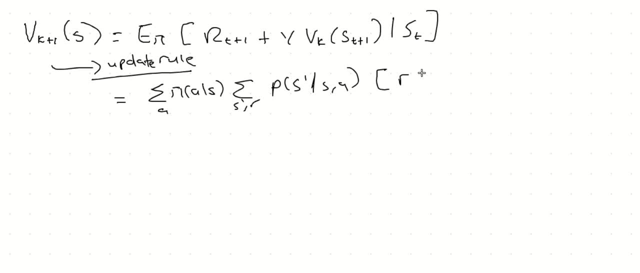 our transition probability, R plus gamma VK of s prime. so again, this kind of formulation we have is that the value of VK plus 1 is actually depending on, now, the value of VK. okay, so we're looking at the previous value and so forth. so this is what we call the expected update. that's another name. what? 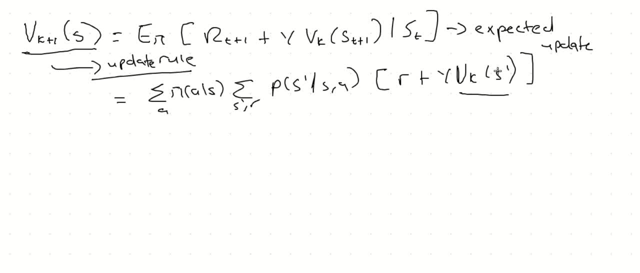 this update rule. okay, so this is kind of like our update rule for a given state. okay, so this is kind of like our update rule for a given state. okay, so this is kind of like our update rule for a given state, showing this kind of value iteration problem: sorry, a policy iteration. so now that we've reached this, 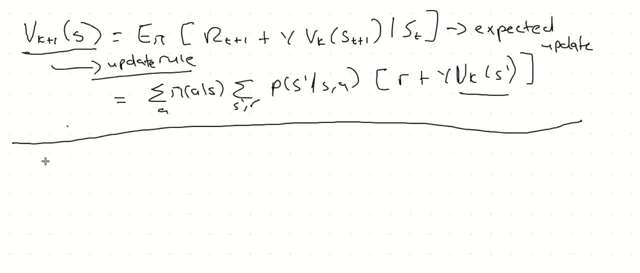 point right. I should also mention a key point that I'm going to just write down: the basic algorithm for solving the policy evaluation problem using this update rule. so this algorithm, and actually most of the material that I'm covering, is actually in a book by our L, by. 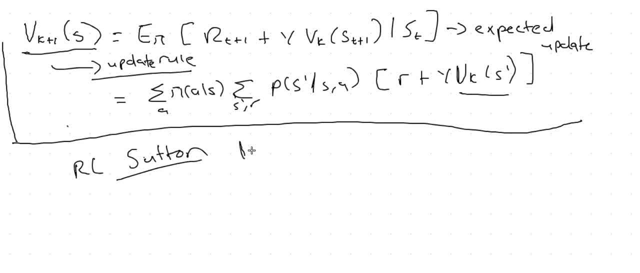 Sutton introduction to reinforcement learning. so if you search for Sutton's book- and you should be able to see this stuff in more detail- I'm just trying to cover and explain the concepts that are actually illustrated in here, and I'm going to add, of course, programming exercises and so forth for this. so let's go through. 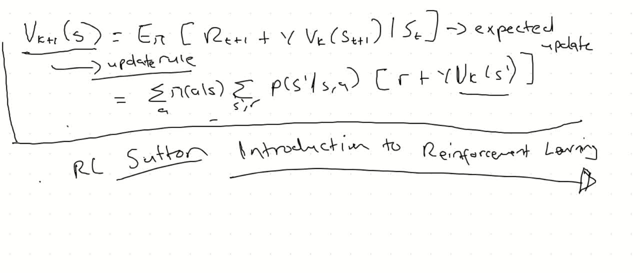 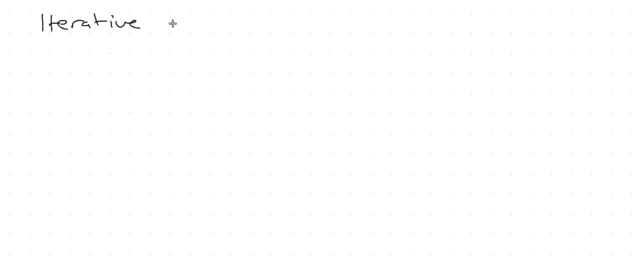 our software policy evaluation algorithm, the iterative- so this should be good for the programmers, I guess. iterative policy evaluation. so what was the first thing we assumed? we are actually given a the policy, right, someone gave us this policy and they want us to evaluate this policy. so this is our policy to be evaluated, right? 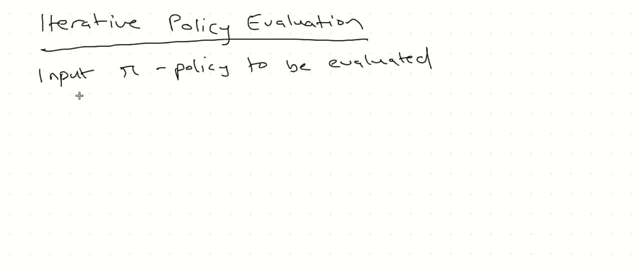 so the first thing we need to do, right is we need to initialize an array: right vs, the value for all the states. right, so vs is close to zero for all. s is an element of s, which is our, i will say, capital. s like this is our state space actually. so this is our state space. 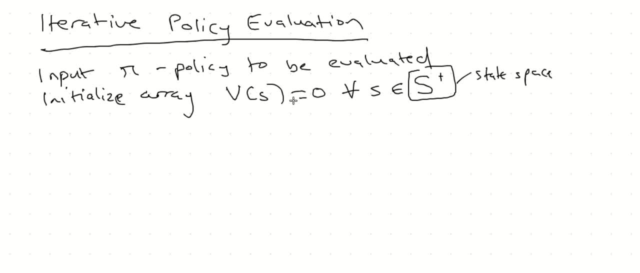 so we initialize the values for each state in the beginning to be equal to zero, and after that we're going to repeat the following: right, so we start by some delta. we initiated to be equal to zero. this is for convergence properties, but we'll go to it now for each state. 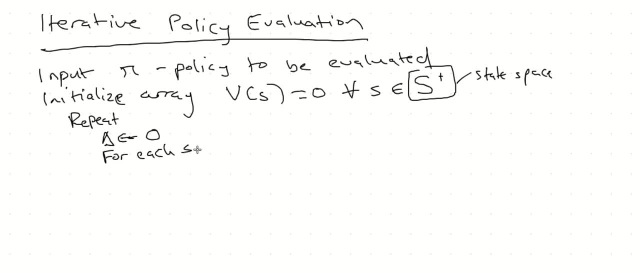 for each state. s is an element of s right. what we want to do right is to assign right v right. what are we assigning v to? v is equals to vs. okay, some v is equals to vs: the value of that state. and then what is vs? well, we know what vs is. we know the update rule. 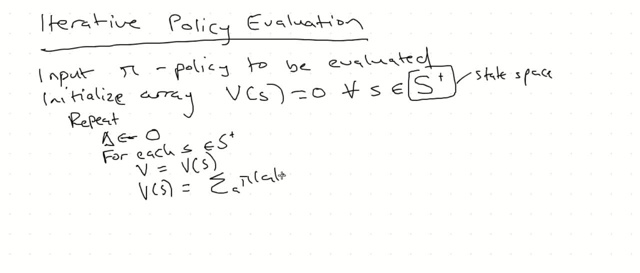 is the summation over a of pi a given s times, summation over s prime comma r of ps prime comma r, even s comma a. again, this is interchangeable with this, in case you forgot. like this, we're just saying: this is the same thing and multiply this by r plus gamma times v.